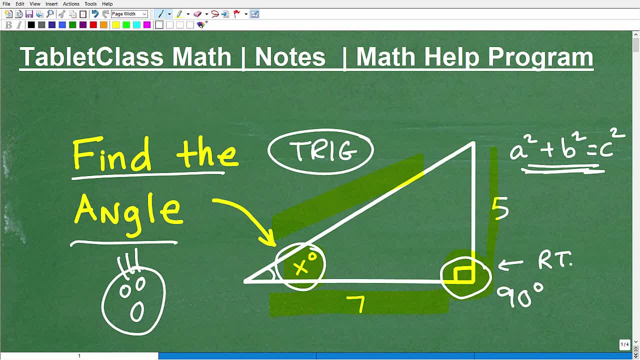 You know it's so advanced. Now listen, you've got to relax, right? This stuff does not have to be scary, And what we're going to be talking about here is basic, basic trigonometry, to include the sine, cosine and tangent functions or trigonometric ratios, And we're going to use one of these guys. 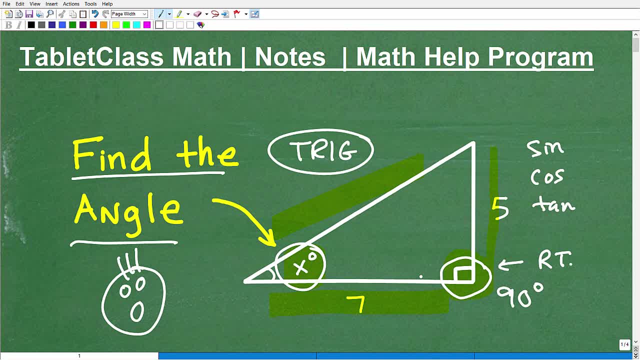 here to solve this problem. So if you are new to trigonometry, stick around. I think you'll find this interesting. But you know, if you're studying problems like this, well then obviously you're already probably using basic trigonometry. Now, if you want to kind of play along and do the 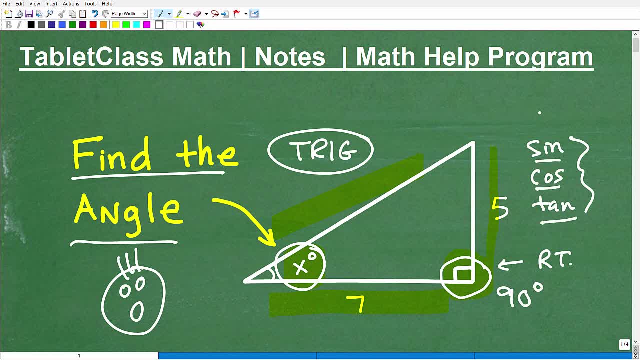 problem on your own. you will need a scientific calculator, something that has these buttons on your calculator. That's a scientific calculator. It can be a graphic calculator, but you do need these basic trigonometric functions, And I'm going to get into all of. 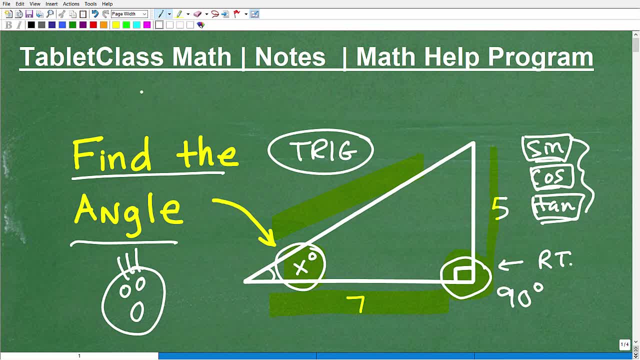 this in just one second, But first let me quickly introduce myself. My name is John. I'm the founder of Tablet Class Math. I'm also a middle and high school math teacher And over several years I've constructed what I like to believe is one of the best online math help programs there is. 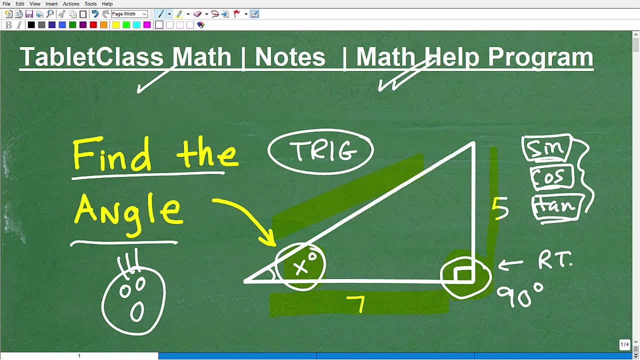 Of course I'll let you be the judge of that. You can check out my math help program at the link in the description of this video. But basically I have 100 plus different math courses. I have all the main courses like pre-algebra, algebra one, geometry, algebra two. I'm going to be launching. 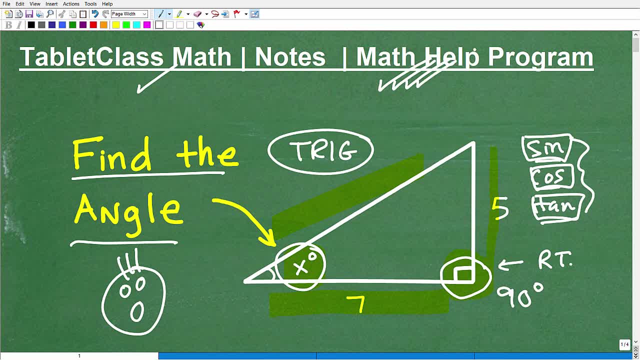 pre-calculus here shortly, But I have a lot of courses in the area of test preparation, so if you're studying for the GED, SAT, ACT, GRE, GMAT, maybe the CLEP exam, ACCUPLACE or ALEKS. 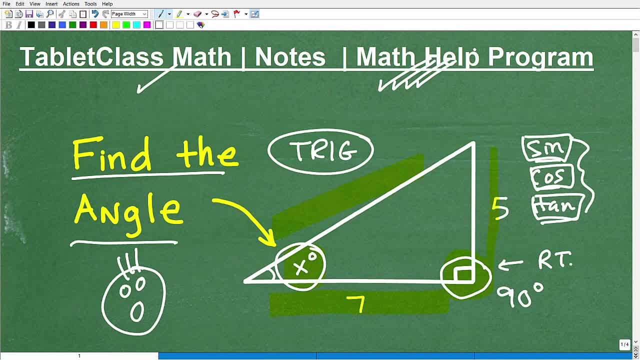 teacher certification, like a practice exam, or nursing entrance TEAS. there's so many exams out there that people have to take that involve a lot of math, And if you don't get to the math section on these particular exams, you don't pass the exam and that has serious consequences. So 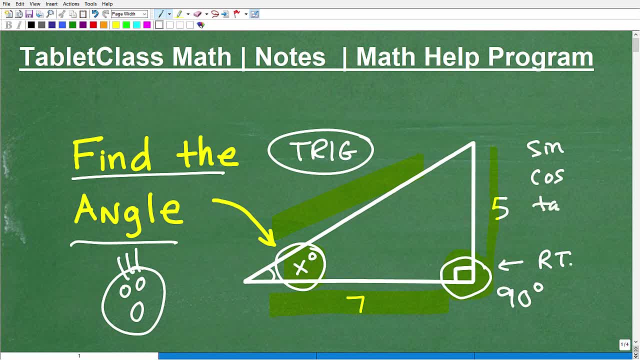 the sine, cosine and tangent functions, or trigonometric ratios, And we're going to use one of these guys here to solve this problem. So if you are new to trigonometry, stick around. I think you'll find this interesting. But you know, if you're studying problems like this, well then. 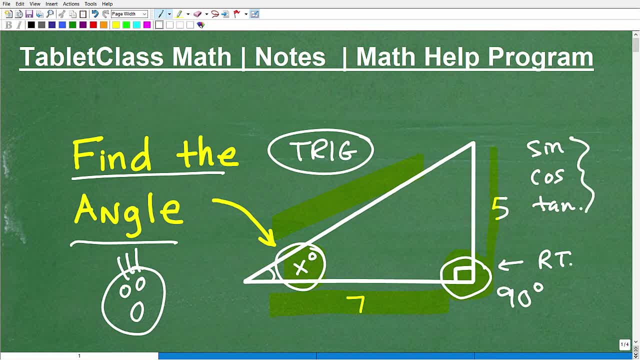 obviously you're already probably using basic trigonometry. Now if you want to kind of play along and do the problem on your own, you will need a scientific calculator, something that has these buttons on your calculator. That's a scientific calculator. It can be a graphic. 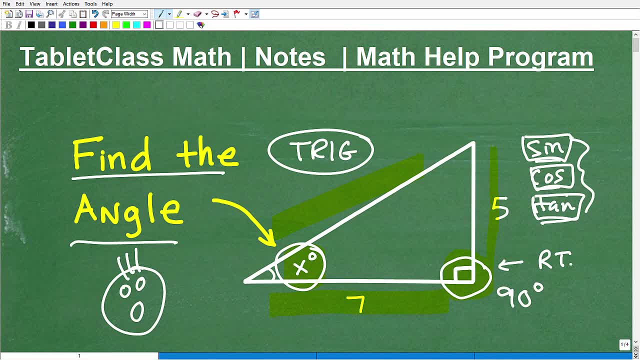 calculator, but you do need these basic trigonometric functions, And I'm going to get into all of this in just one second. But first let me quickly introduce myself. My name is John. I'm the founder of Tablet Class Math. I'm also a middle and high school math teacher, and 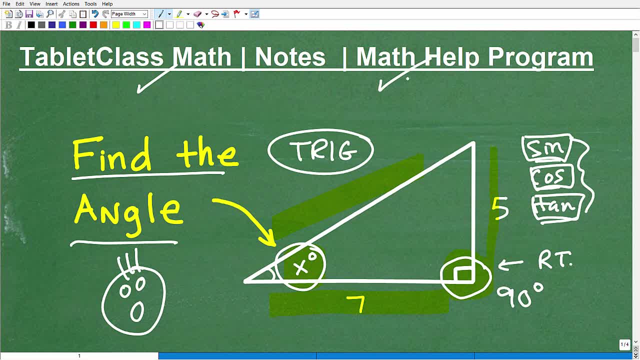 over several years I've constructed what I like to believe is one of the best online math help programs there is. Of course, I'll let you be the judge of that. You can check out my math help program at following the link in the description of this video. But basically I have 100 plus. 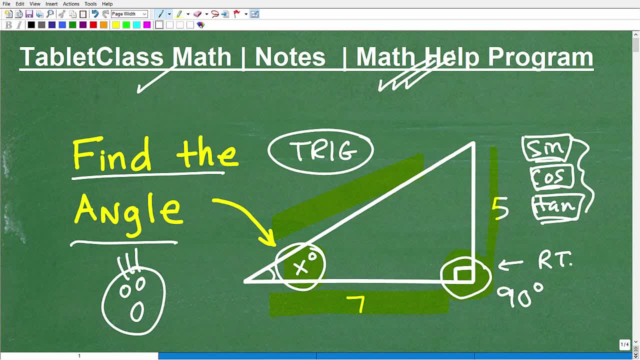 different math courses. I have all the main courses like pre-algebra, algebra one, geometry, algebra two. I'm going to be launching pre-calculus here shortly, but I have a lot of courses in the area of test preparation. So if you're studying for the GED, SAT, 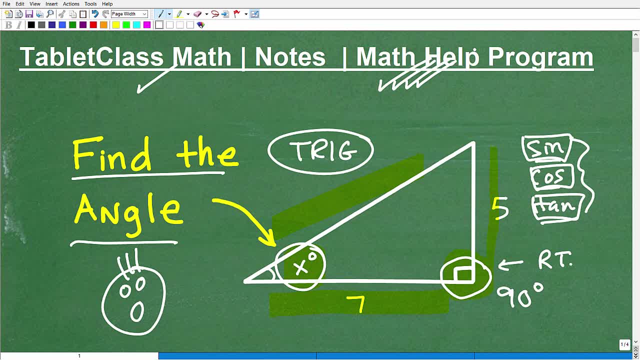 ACT, GRE, GMAT, maybe the CLEP exam, ACCUPLACE or ALEKS, teacher certification, like a practice exam, or nursing entrance, TEAS. there's so many exams out there that people have to take that involve a lot of math, And if you don't get to the math section on these particular exams, you don't pass. 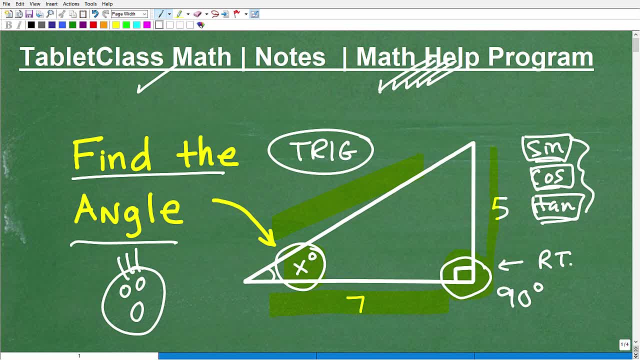 the exam and that has serious consequences. So if you're studying for any of these exams, just go to my site. I should have you. go to my course catalog. I should have the exam you're looking for, If I don't, drop me a line and I'll help you out the best I can. I also do a lot. 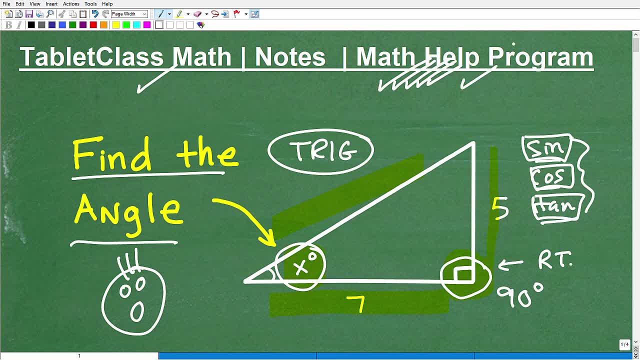 with independent learners like homeschoolers. I have a great homeschool learning system, And then I help those of you who are just struggling in your math class. Now, one thing that I can't do for you, that you must do for yourself, and that is the following: You have to take great math notes. 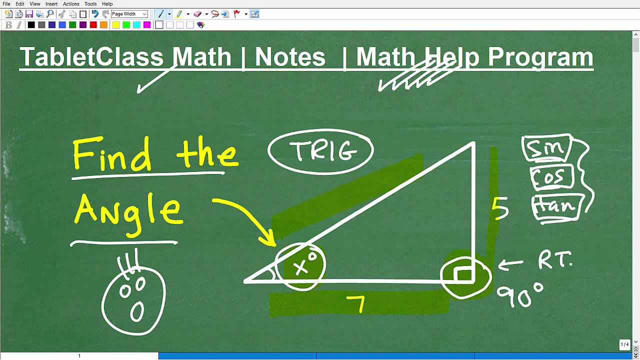 if you're studying for any of these exams, just go to my site. I should have you. go to my course catalog. I should have the exam you're looking for If I don't drop me a line, and I'll help you out the best I can. I also do a lot with independent learners, like homeschoolers. 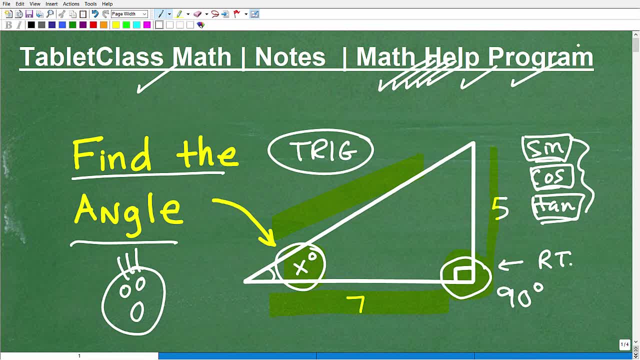 I have a great homeschool learning system, And then I help those of you who are just struggling in your math class. Now, one thing that I can't do for you, that you must do for yourself, and that is the following: You have to take great math notes. So, over decades of teaching, 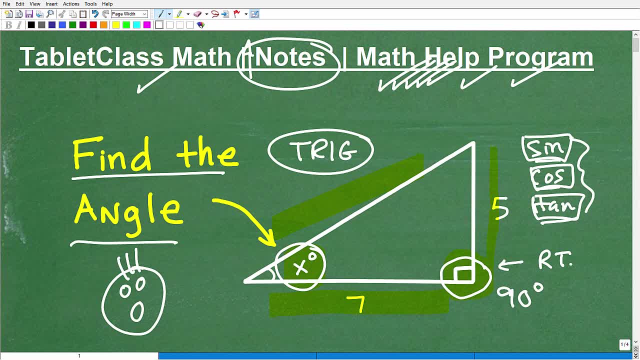 mathematics. one thing is apparent to me: those students who take fantastic math notes almost always do very well in math, And the reverse is true. Those students who think they have this like superpower photographic memory, you know, they're like I can just watch and I'll 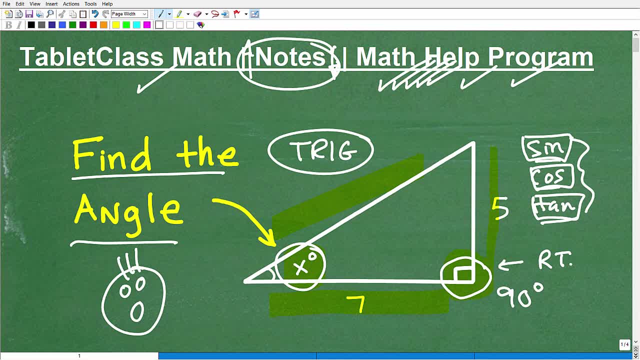 remember everything. They kind of you know, talk themselves into having this superpower. That's not the case. Okay, believe me when I tell you, if you think you have that power, you won't have it for long. in terms of more advanced math, There's just too much information. 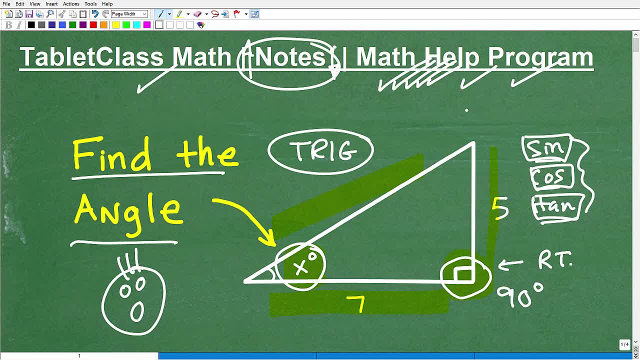 But you know, during class people like to do what? Let's just be honest. They like to look at their cell phone. They like to look at their cell phone. They like to look at their cell phone, They like to talk to their best friend in class And they're like you know what? Their best friend 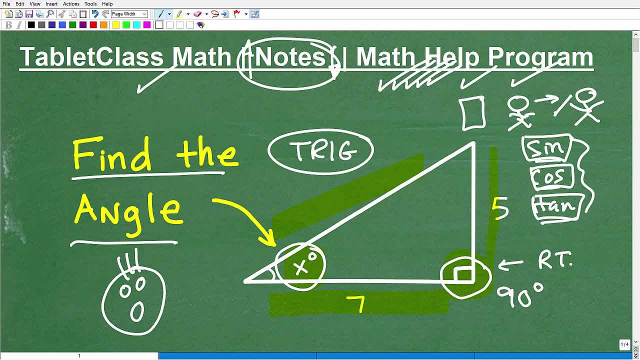 over here is saying, hey, listen, don't talk to me because I'm trying to take notes. And then you say, okay, I won't talk to you because I need you to take the notes, because I'm going to look at your notes. Listen, I did all of that And well, I didn't do the cell phone part back in the 1980s. 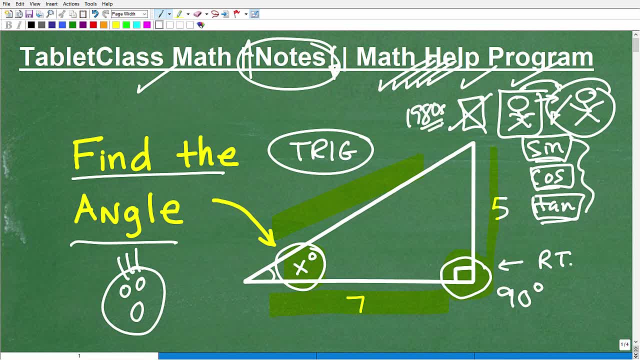 because those guys weren't around, at least not the cool smartphone. So I get that you're totally distracted, Okay, But you, and only you, can fix that situation. And I'm not saying that you can't fix that situation. All right. You have to learn how to focus. Being focused is the key to success. 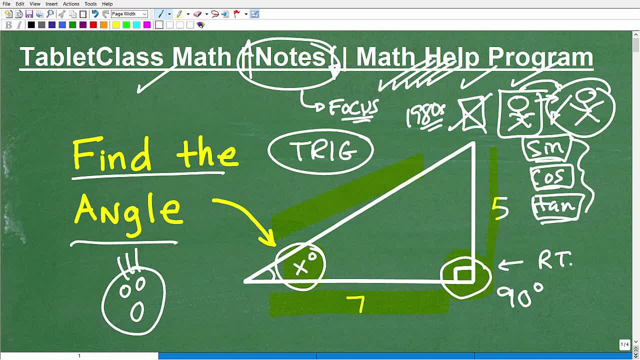 in anything, And the way to keep yourself focused in mathematics is to be engaged in note taking. So try to make your notes like perfect right? If you do that, everything is going to go smooth for you, But in the meantime, you still need something to study from if you don't have great. 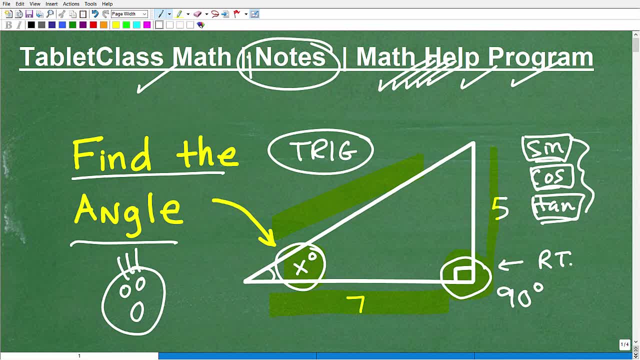 So, over decades of teaching mathematics, one thing is apparent to me: those students who take fantastic math notes almost always do very well in math, And the reverse is true. Those students who think they have this like a superpower photographic memory- you know they're like- 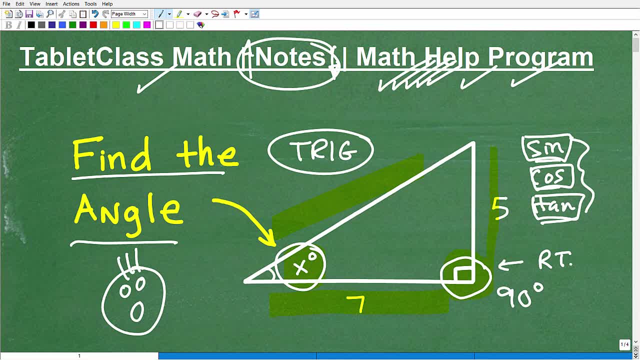 I can just watch and I'll remember everything. They kind of you know talk themselves into having this superpower. That's not the case. Okay, Believe me when I tell you, if you you think you have that power, you won't have it for long. in terms of more advanced math, There's just too much. 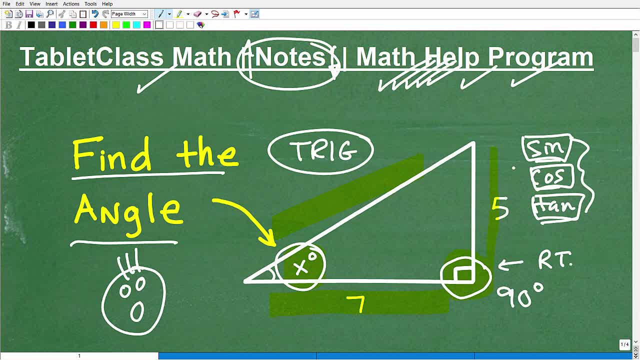 information. But you know, during class people like to do what? Let's just be honest. They like to look at their cell phone, They'd like to talk to their best friend in class And they're like you know what Their best friend over here is saying: hey, listen, don't talk to me, because 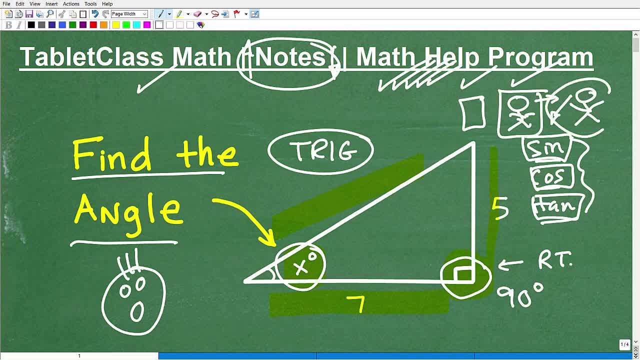 I'm trying to take notes And then you say, okay, I won't talk to you, because I need you to take the notes, because I'm going to look at your notes. Listen, I did all of that And well, I didn't do. 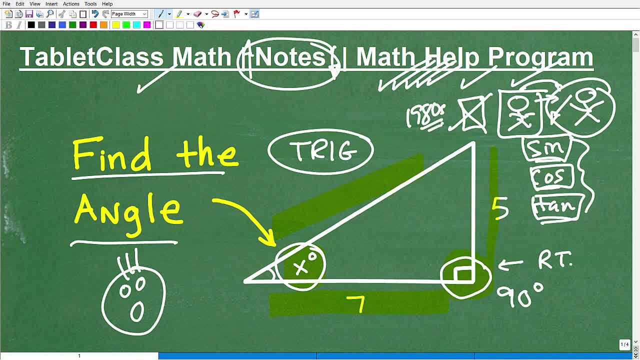 the cell phone part back in the 1980s, because those guys weren't around, at least not the cool smartphones. So I get that you're totally distracted, Okay, But you, and only you, can fix that situation. All right, You have to learn how to focus. 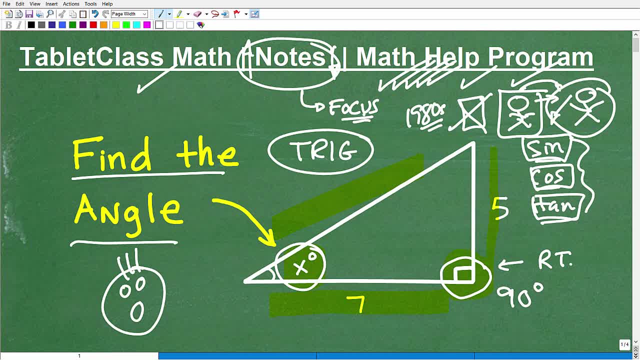 Being focused is the key to success in anything, And the way to keep yourself focused in mathematics is to be engaged in note-taking. So try to make your notes like perfect right. If you do that, everything is going to go smooth for you, But in the meantime, you still need something to study. 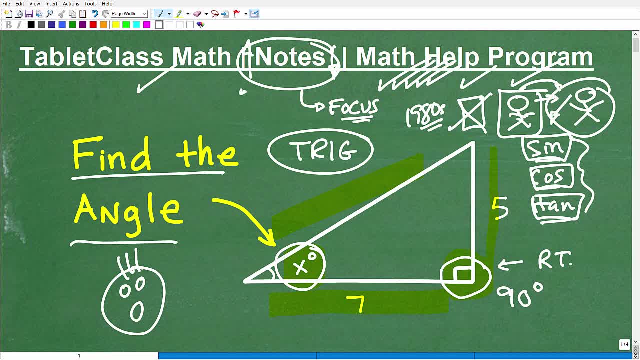 from if you don't have great notes right now. So I offer notes to include pre-algebra, algebra one, geometry, algebra two and trigonometry. You can find links to those notes in the description of this video. Okay, So if you're interested in learning more about math, you can go to. 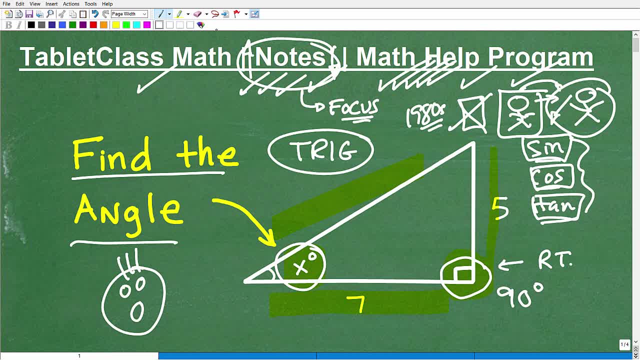 If you want to try this problem on your own. of course it's kind of scribble scratch right here, but here is the problem. You'll need a calculator, but go ahead and pause the video if you want to go ahead and give this a try on your own. I'm going to get into this now, Okay, So if you don't want, 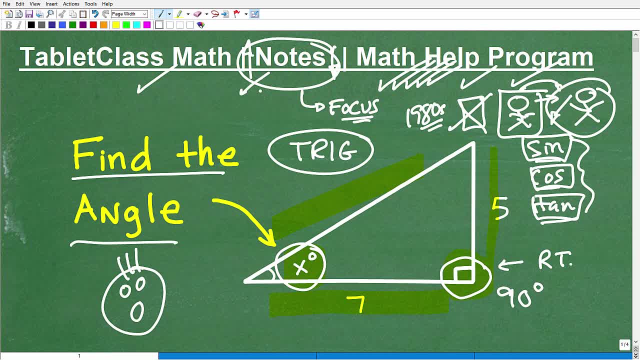 notes right now. So I offer notes to include pre-algebra, algebra one, geometry. algebra two, trigonometry. You can find links to those notes in the description of this video. Okay, So if you want to try this problem on your own, of course it's kind of a scribble, scratch right here. 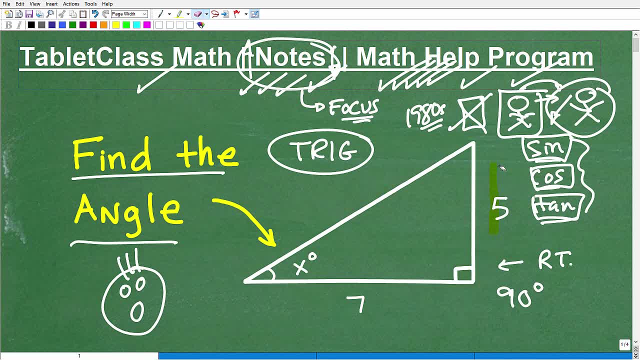 but here is the problem. You'll need a calculator, but go ahead and pause the video if you want to. go ahead and give this a try on your own. I'm going to get into this now, Okay, So if you don't want, 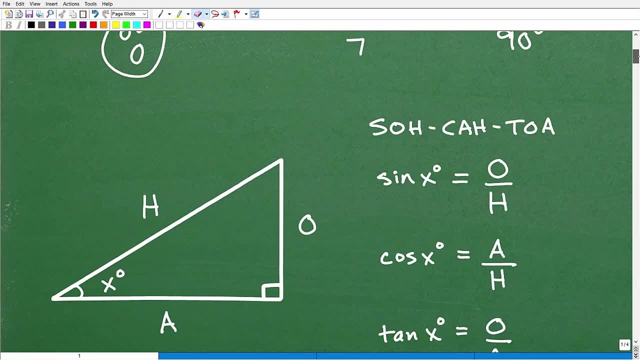 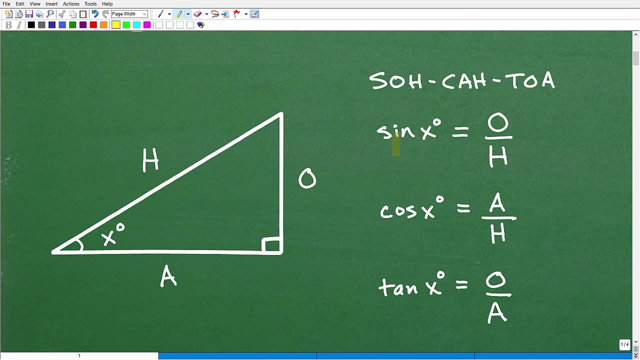 to see the solution, pause the video. but let's talk first about basic trigonometry. Okay, So what are we going to need here to solve this problem? Well, we're going to need to have a basic understanding of something called these trigonometric functions, called sine cosine. 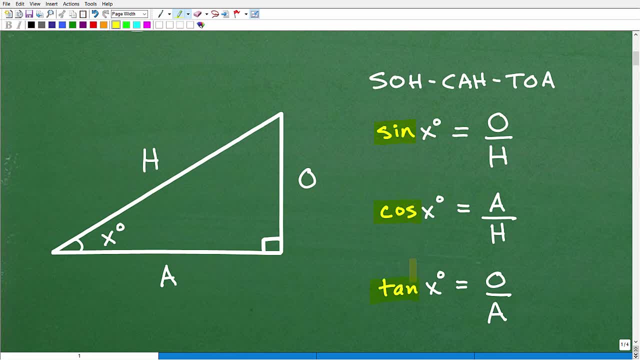 and tangent. These are the basic trigonometric functions. We call them trigonometric ratios as well. And here I have a little saying. okay, it's super famous saying: I bet your grandparents learned this back in high school, way back in the good old days. It goes like this: So Katoa. 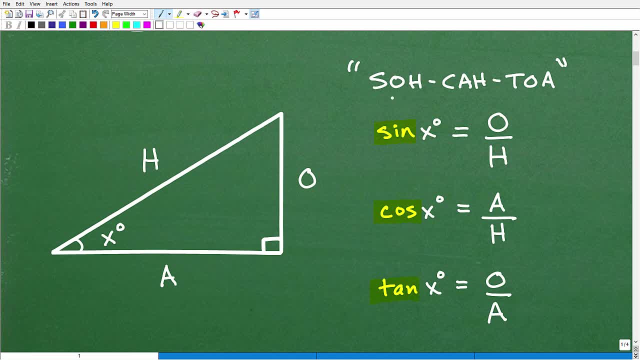 and you might be saying, oh okay, I don't even know what this guy's talking about. Well, what this stands for is so it stands for: the sine is equal to the opposite over hypotenuse, Cosine is the adjacent over the hypotenuse and tangent is the opposite over the adjacent. So 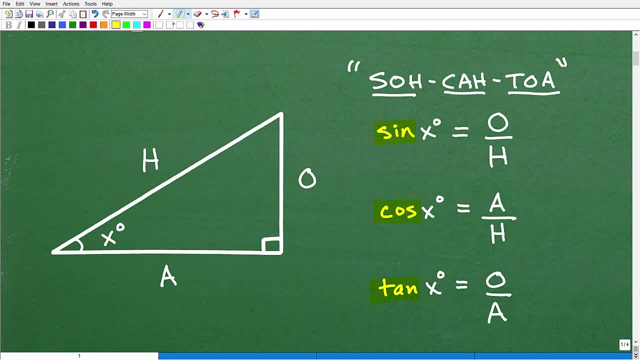 let's kind of put some definition on this right now. So here is our angle. Okay, Well, we're looking at a right triangle. We can kind of define the sides of this triangle Now. in a right triangle, the longest side, okay, The longest side of the right. 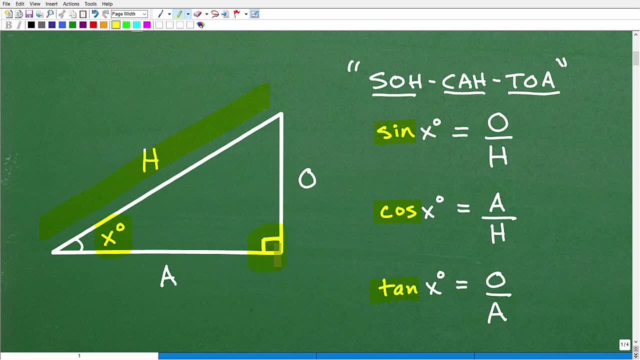 triangle and that's going to be opposite of the 90 degree angle. Okay, It should be obvious. This is the longest side. This is H. Okay, This is called the hypotenuse. All right, Now, here is our angle: the leg or the side that's next to the angle. Okay, Right here, This is called the. 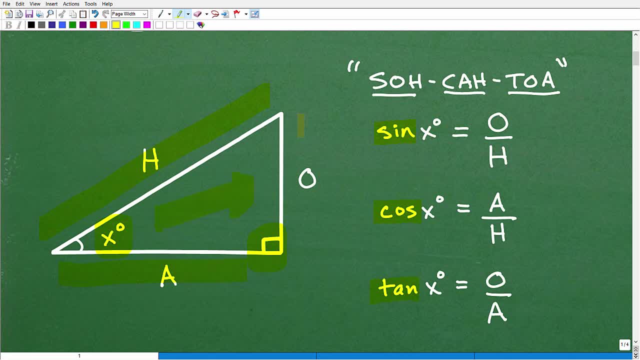 adjacent side And then the side opposite of that angle is called the opposite Side. Okay, So, anytime you're looking at an angle, you'll be able to determine the opposite side, the adjacent side and the hypotenuse in terms of a right triangle. Okay, So let's go. 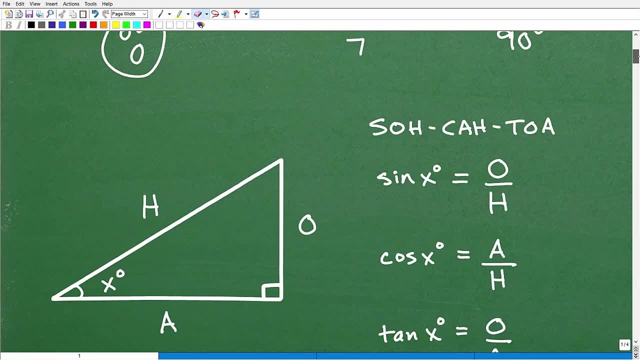 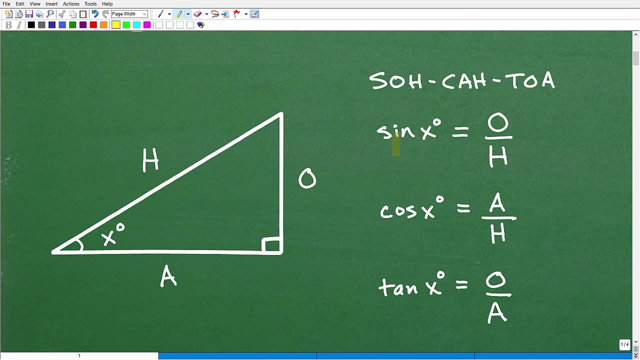 to see the solution, pause the video. but let's talk first about basic trigonometry. Okay, So what are we going to need here to solve this problem? Well, we're going to need to have a basic understanding of something called these trigonometric functions, called sine cosine. 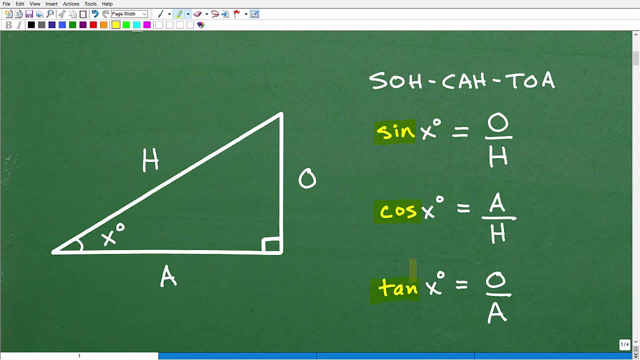 and tangent. These are the basic trigonometric functions. We call them trigonometric ratios as well. And here I have a little saying. Okay, It's super famous saying: I bet your grandparents learned this back in high school, way back in the good old days. It goes like this: So: 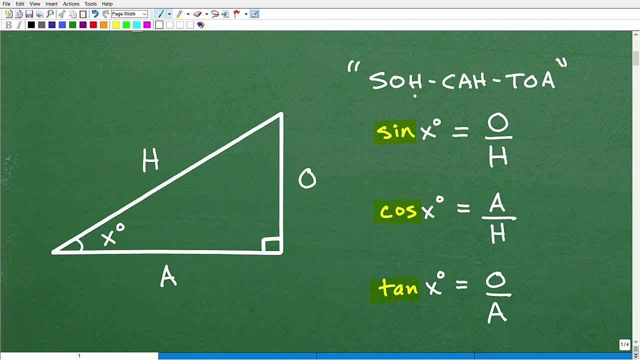 Katoa and you might be saying, oh okay, I don't even know what this guy's talking about. Well, what this stands for is so it stands for the sine is equal to the opposite. over hypotenuse Cosine is the adjacent. 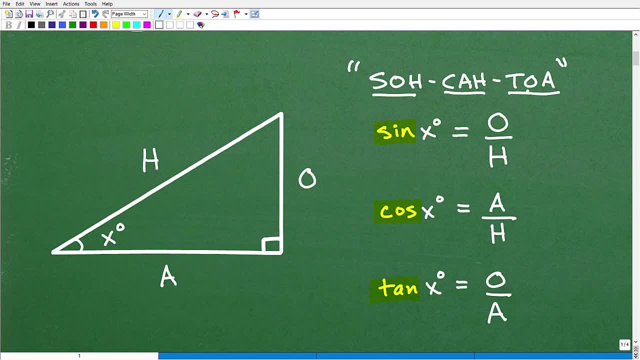 over the hypotenuse, and tangent is the opposite over the adjacent. So let's, let's kind of put some definition on this right now. So here is our angle. Okay, When we're looking at a right triangle, we can kind of define the sides of this triangle. Now, in a right triangle, the longest- 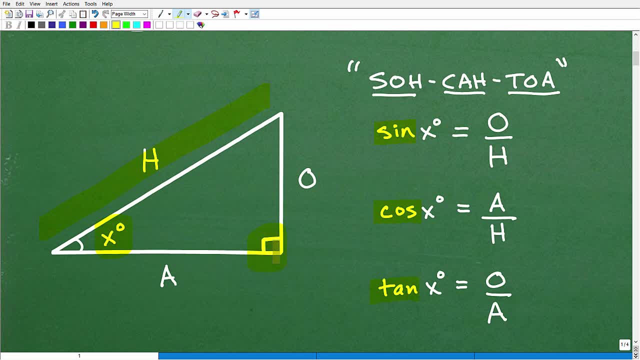 side of the right triangle and that's going to be opposite of the 90 degree angle. Okay, It should be obvious. This is the longest side. This is H. Okay, This is called the hypotenuse. All right, Now, here is our angle, the leg or the side that's next to the angle. Okay, Right here. 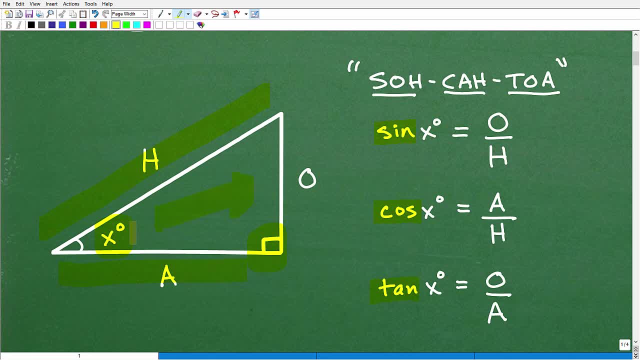 this is called the adjacent side, And then the side opposite of that angle is called the opposite side. Okay, So anytime you're looking at an angle, you'll be able to determine the side, the adjacent side and the hypotenuse in terms of a right triangle. Okay, So let's go back. 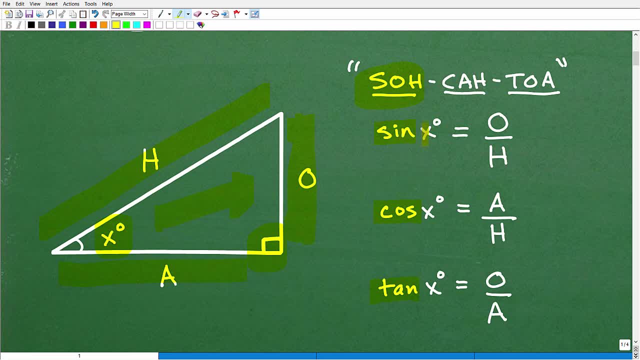 to this little saying: SOH, CAH, TOA. So the sine of angle X will be equal to OH, opposite, this one over the hypotenuse. Okay, So this is the opposite. That's the hypotenuse. So that's what. 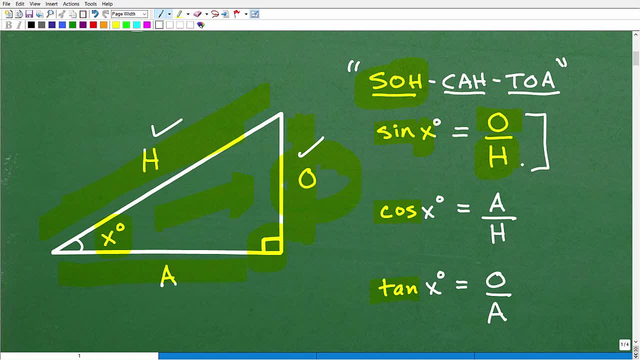 the, the sine of that angle is defined as All right. This is why we call these trigonometric ratios, because the ratio is just basically a comparison of two, two values. Okay, A fraction, if you will. Okay, So in here we have cosine. Cosine would be the adjacent over the hypotenuse. 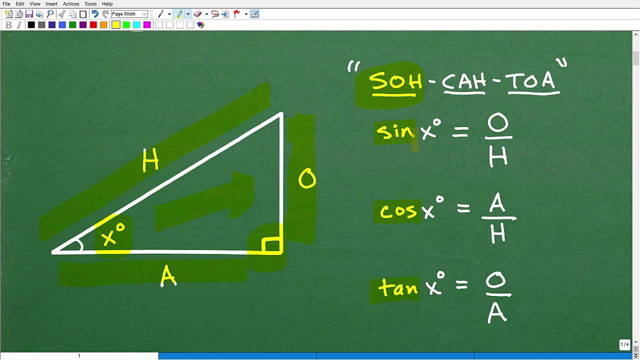 back to this little sayings: So Katoa, So the sine of angle X will be equal to O H, opposite, this one over the hypotenuse. Okay, So this is the opposite. That's the hypotenuse. So that's what. 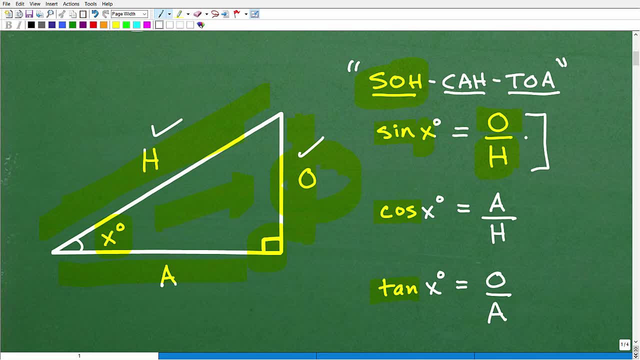 the sine of that angle is defined as All right. This is why we call these trigonometric ratios, because the ratio is just basically a comparison of two, um, uh, two values. Okay, A fraction, if you will. Okay, So in here we have cosine. Cosine would be the adjacent. 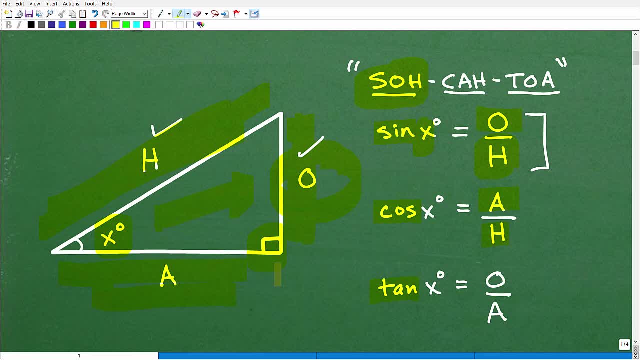 over the hypotenuse. So if I had the actual um, uh legs, okay, If this was- let's use an easy one here- a three, four, five right triangle, And these are actual uh lengths, We can kind. 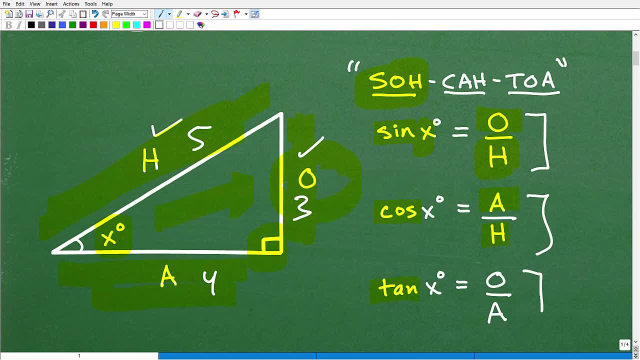 of you know, calculate these out and then tangent is equal to the opposite over the adjacent. Okay, All right. Now these are our, uh kind of our, options here. We have the sine, the cosine and tangent, but, uh, if we can uh use one of these, or we can if we have enough information to. 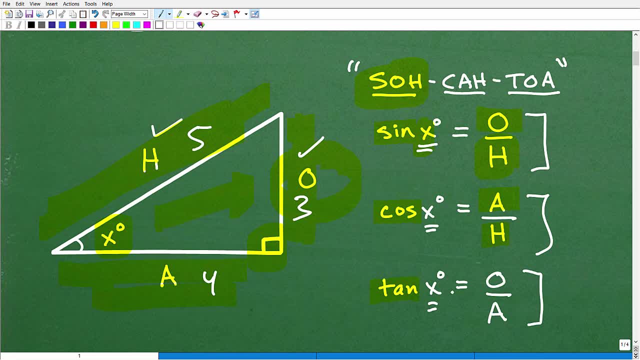 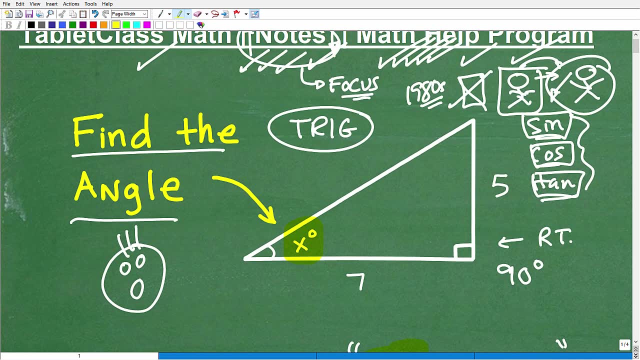 um, use one of these trigonometric functions, then we could solve for the angle. So let's go back to our problem here And let me ask you: what sides do we have? I have this angle, but I have this side and this side. So what are those sides? Well, 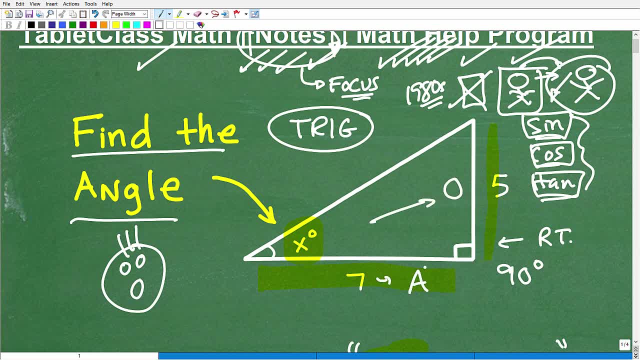 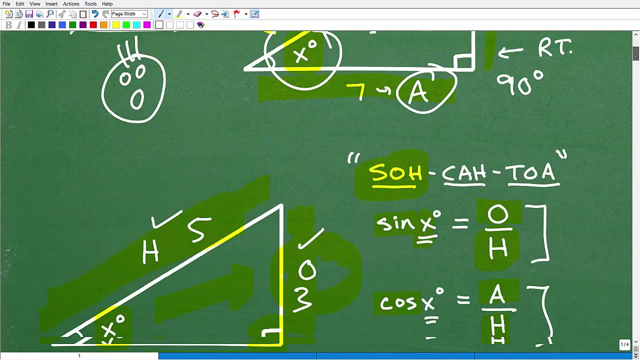 this is the opposite and this is the adjacent. So I'm going to need to use the trigonometric function that involves the opposite and the adjacent. And now let's go take a look at our options, which one involves the opposite and the adjacent? And if you said tangent, I would say: 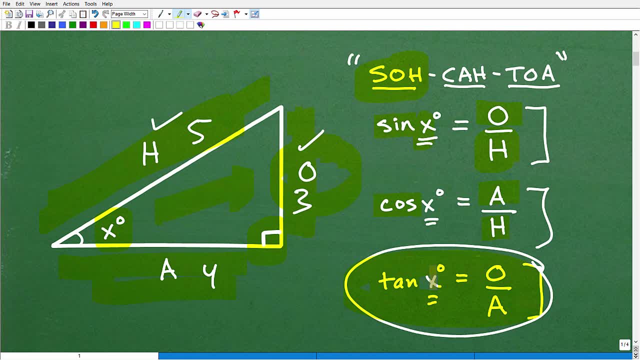 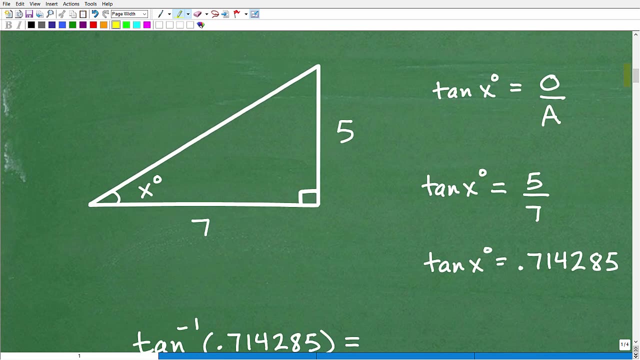 fantastic, You're paying attention, And that is exactly right. We need to use the tangent. Okay, So the tangent is TOA. It's defined as the opposite over the adjacent. Now, with the armed with that information, let's get to the problem. Okay, So, uh, now again, we're going to use the tangent, so we can. 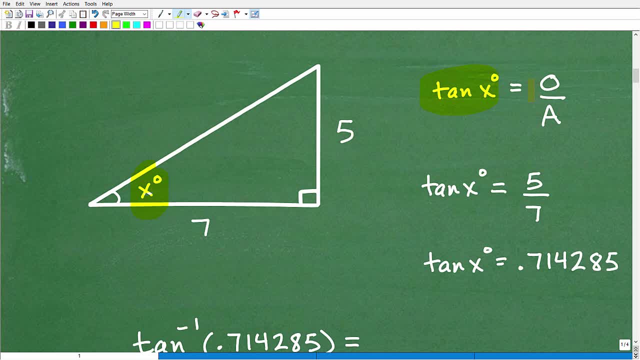 say the tangent of this angle is going to be equal, to remember TOA, T O A, the opposite. So that's five. Okay, That will be this. uh, that's the going to be the opposite value here in a second, And then the Jason. 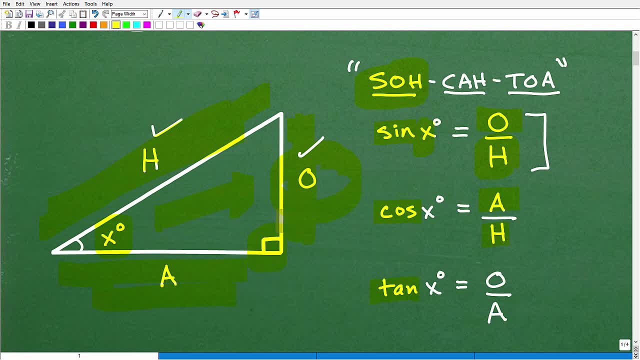 So if I had the actual legs, okay, if this was- let's use an easy one here- a three, four, five right triangle, and these are actual lengths. we can kind of, you know, calculate these out, And then tangent is equal to the opposite. 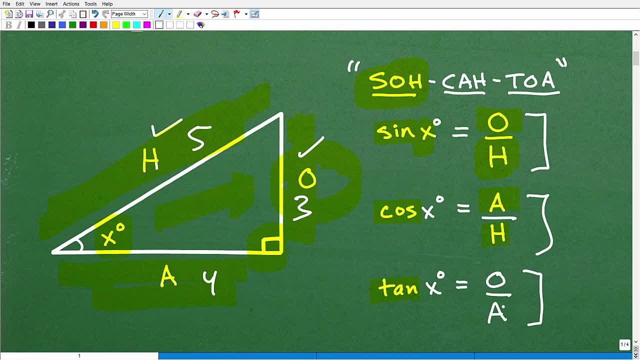 Over the adjacent. Okay, All right. Now these are our kind of our options. here We have the sine, the cosine and tangent, but if we can use one of these, or we can, if we have enough information to use one of these trigonometric functions, then we could solve for the angle. 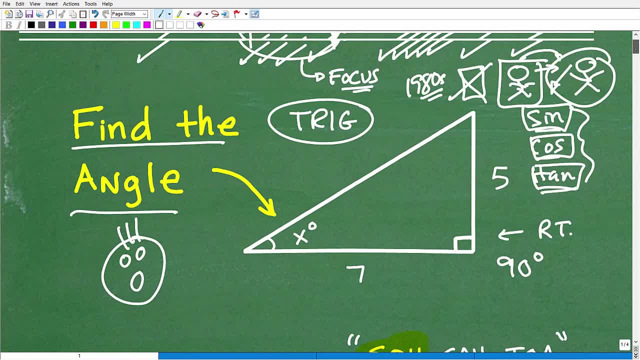 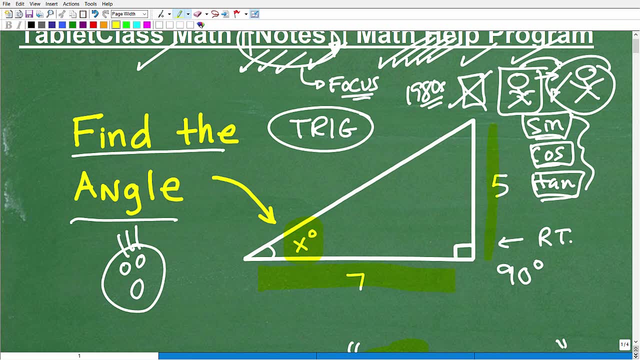 So let's go back to our problem here And let me ask you: what sides do we have? I have this angle, but I have this side and this side. So what are those sides? Well, this is the opposite and this is the adjacent, So I'm going to need to use the trigonometric. 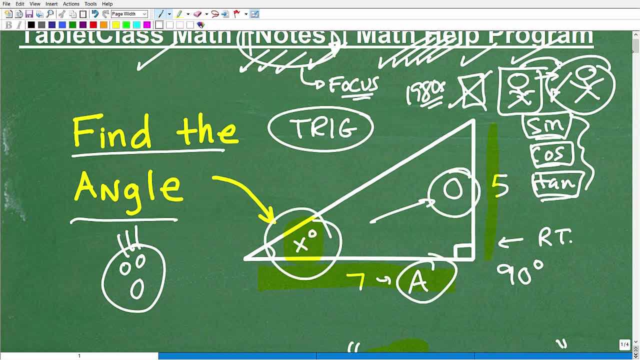 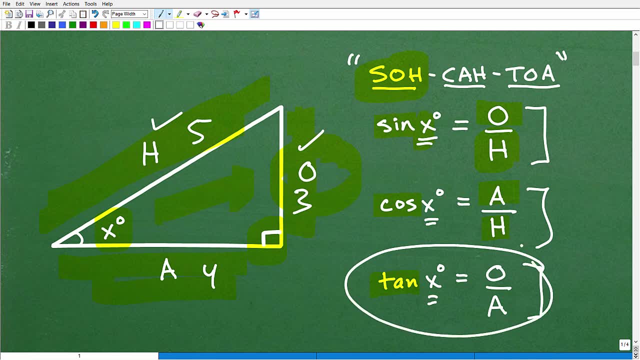 function that involves the opposite and the adjacent. And now let's go take a look at our options, which one involves the opposite and the adjacent. And if you said tangent, I would say fantastic, You're paying attention, And that is exactly right. We need to use the tangent, Okay. 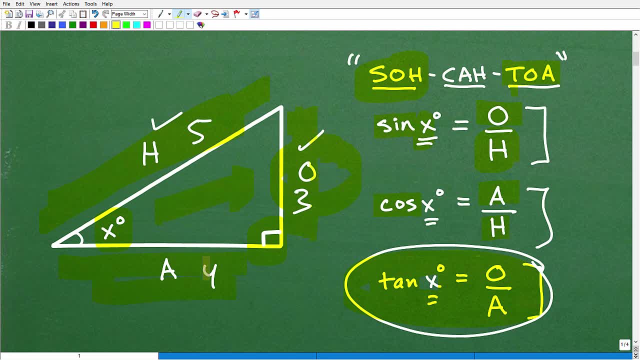 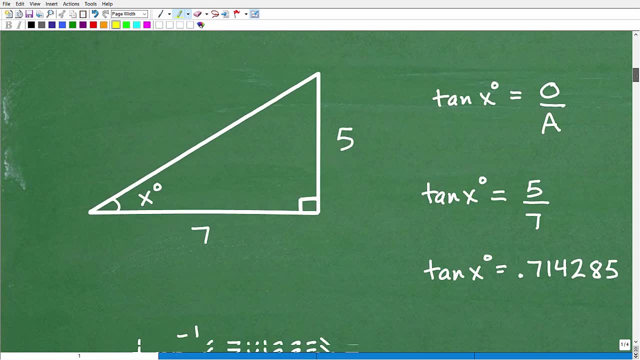 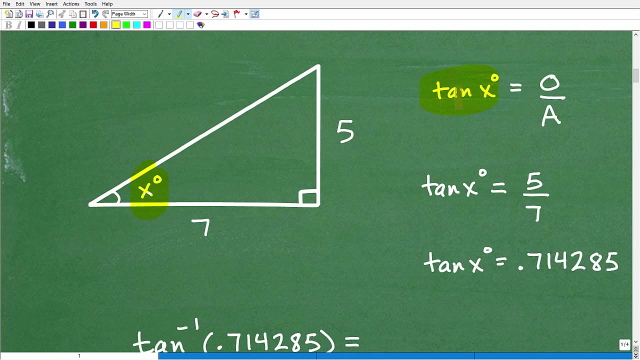 So the tangent is TOA. It's defined as the opposite, over the adjacent. Now with the armed formation, let's get to the problem, Okay, So now again, we're going to use the tangent So we can say: the tangent of this angle is going to be equal, to remember: TOA, T-O-A, the opposite. So that's. 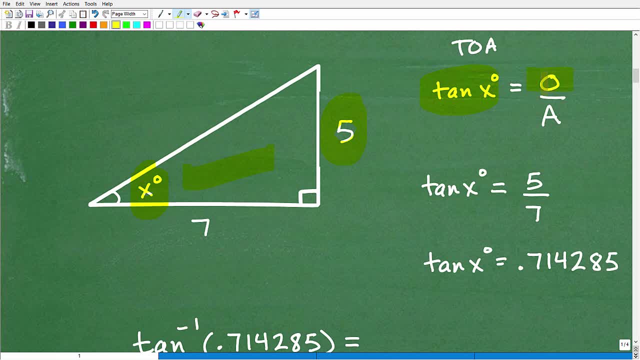 five. Okay, That will be this. That's going to be the opposite value here in a second, And then the adjacent is seven. Okay, So let's go ahead and plug this in. So the tangent of this angle here is five over seven. So you know how is this going to help us find the angle? Well, I'm going. 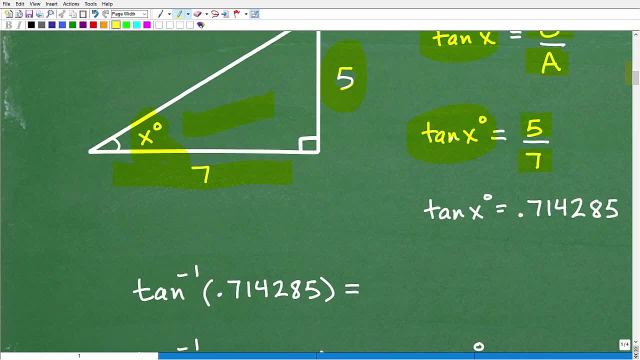 to show you this now. So go into your little calculator and take five and divide it by seven. You're going to get a decimal. and I'm going to kind of round it off here. You're going to get: five divided by seven is going to be 0.714285.. This continues on, but let's just go ahead and 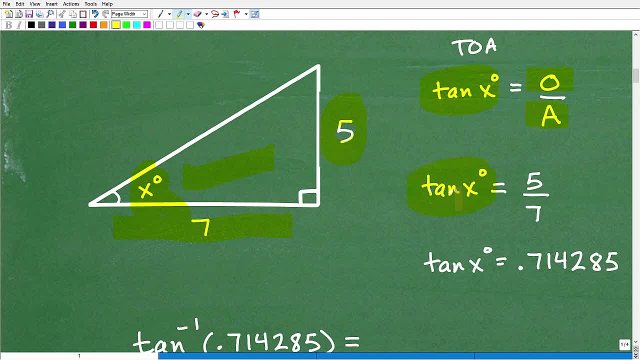 7, okay, so let's go ahead and plug this in. so the tangent of this angle here is 5 over 7. so you know how is this going to help us, uh, find the angle? well, i'm going to show you this now, so go into. 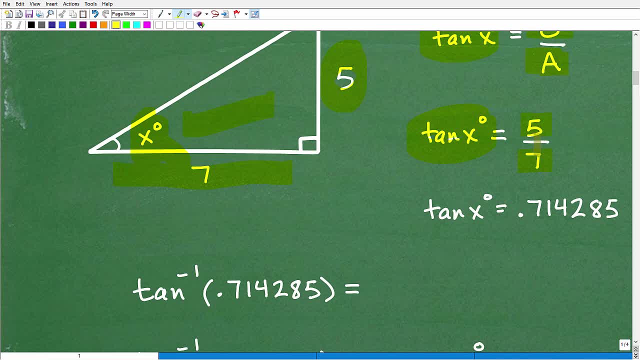 your little calculator and take 5 and divide it by 7, you're going to get a decimal. and i'm going to kind of round it off here. you're going to get 5 divided by 5. divided by 7 is going to be 0.714285. 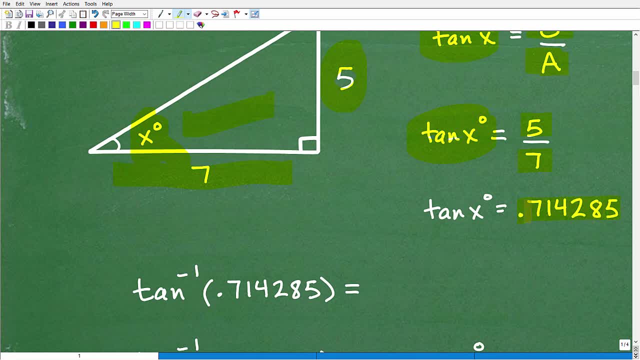 this continues on, but let's just go ahead and stop it with these, uh, six digits. now a couple things you need to know: the the more digits i write of this value, uh, the more accurate my answer will be: okay, that's just kind of. you don't want to use like 0.7 or 0.714 put in. you know, i would. 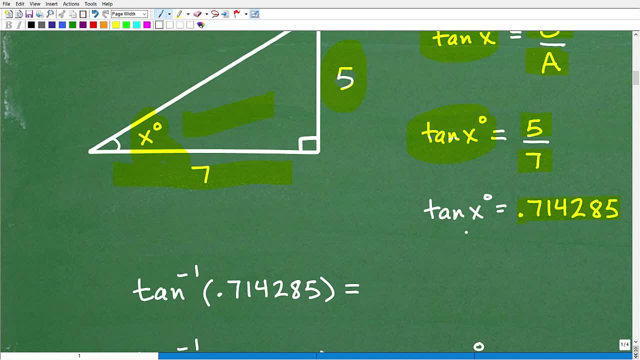 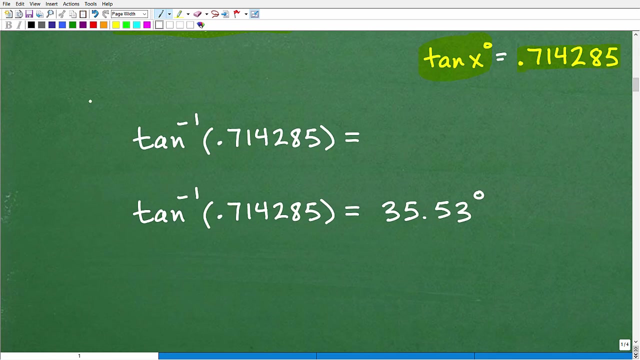 say a good amount of digits, maybe at least six digits, to get the most accurate answer. all right, so we're saying the tangent of this angle here- okay, whatever it is- is 0.714285. now we have to use our calculator to ask a question. okay, now here's the question we're going to ask our calculator. we're going to say, all right, mr. 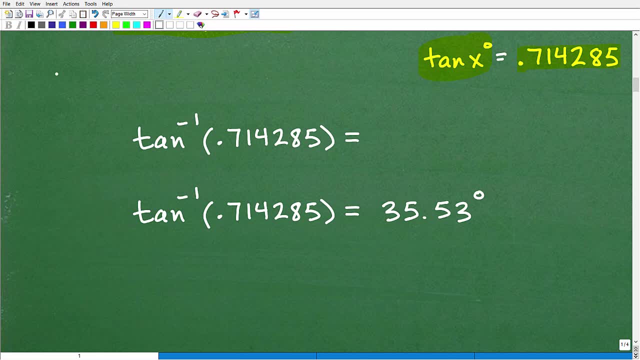 calculator, tell me the angle, what angle? i'll write it out here: what angle has a tangent equal to 0.714285? 0.714285, okay, it's because if i can find that angle right, what angle has a tangent that's equal to 0.714285? because this angle here i'm like all right, mystery angle. i know you, i don't know your. 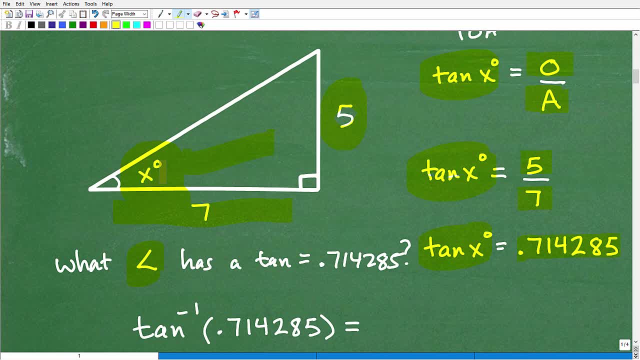 actual angle measure yet, but i do know that your tangent is 0.714285. so you know, i'm going to figure you out, uh, what i'm trying to, you know, uh, answer the question is: what angle has a tangent equal to 0.714285? well, this is where you need to. 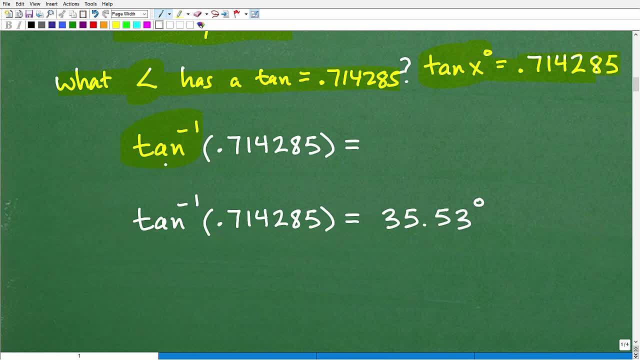 use the arc tangent. okay, it looks like this: um, it's a little tangent with a negative one, and each one of these trigonometric functions has this. so you can have the sine, arc sine, you can have arc cosine, like that, and then you can have arc tangent. now the way you get to this on your calculator. 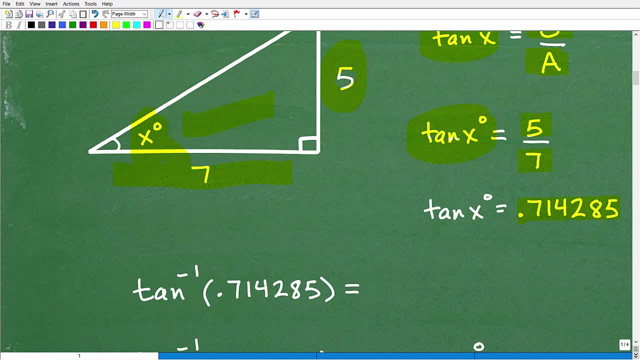 stop it with these six digits. Now a couple of things you need to know. The more digits I write in value, the more accurate my answer will be: Okay, That's just kind of. you know. you don't want to use like 0.7 or 0.714.. Put in, you know, I would say a good amount of digits, maybe at least. 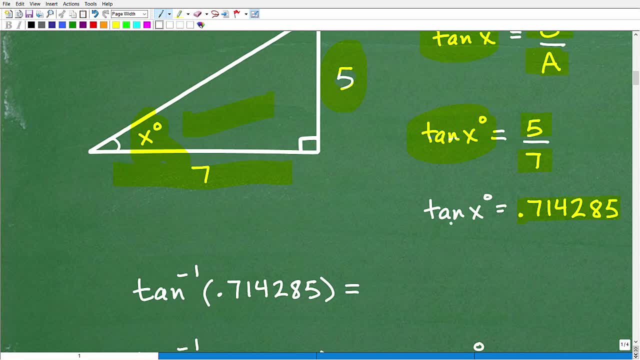 six digits to get the most accurate answer. All right, So we're saying: the tangent of this angle here- okay, whatever it is- is 0.714285.. Now we have to use our calculator to ask a question. Okay, Now here's the question we're going to ask our calculator. We're going to say: 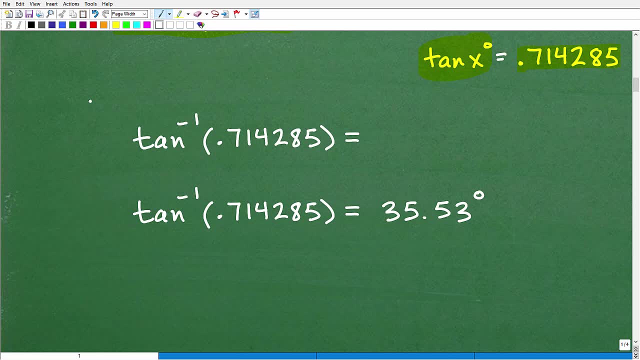 all right, Mr Calculator, tell me the angle, what angle? I'll write it out here: What angle has a tangent equal to 0.714285?? Okay, Because if I can find that angle right, what angle has a tangent that's equal to 0.714285?? 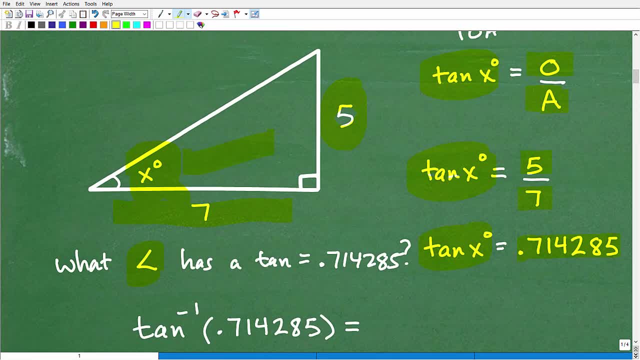 Because this angle here I'm like: all right, Mr Angle, I know you. I don't know your actual angle measure yet, but I do know that your tangent is 0.714285.. So you know, I'm going to figure. 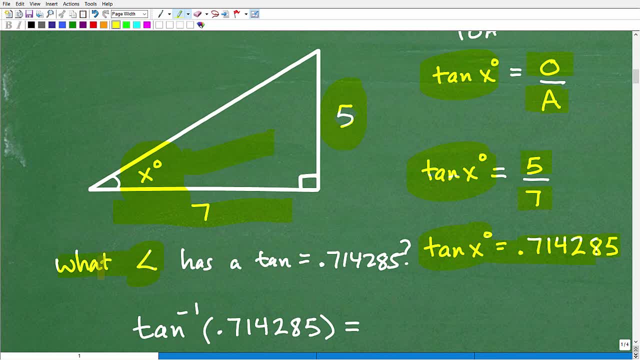 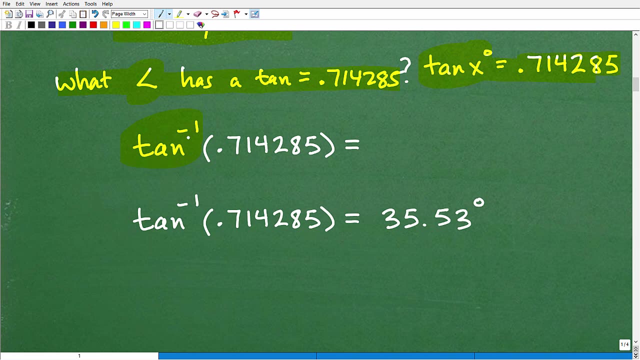 you out What I'm trying to you know answer. the question is: what angle has a tangent equal to 0.714285?? Well, this is where you need to use the arc tangent. Okay, It looks like this: Um, it's a little tangent with a negative one, And each one of these trigonometric functions has. 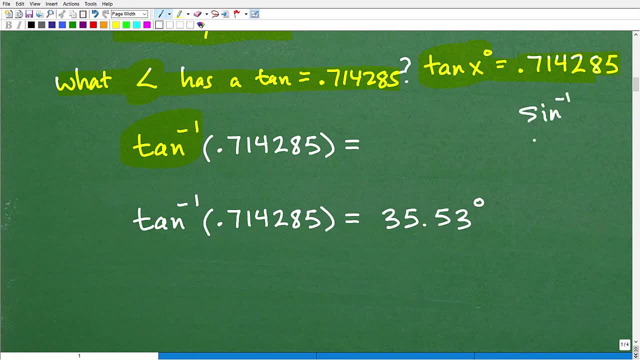 this, So you can have the sine, arc sine, you can have arc cosine like that, and then you can have arc tangent. Now the way you get to this on your calculator is: on your calculator you'll have a tangent button. but you also have a second function on your calculator And if you look like here's: 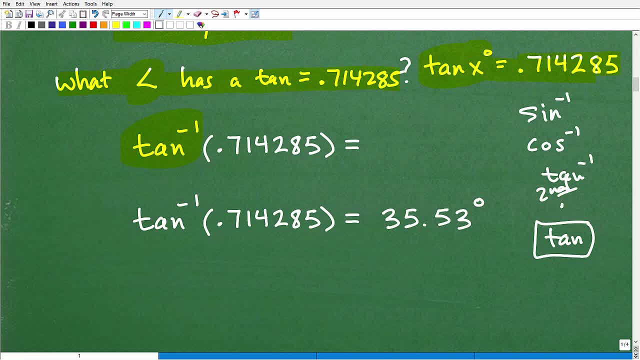 your button, uh, on that, like the face of the calculator, you'll should sit. you should see something like this, So you can have a tangent on your calculator. but you also have a tangent like this. Okay, So you'll have to kind of play with your calculator. You can use these uh. 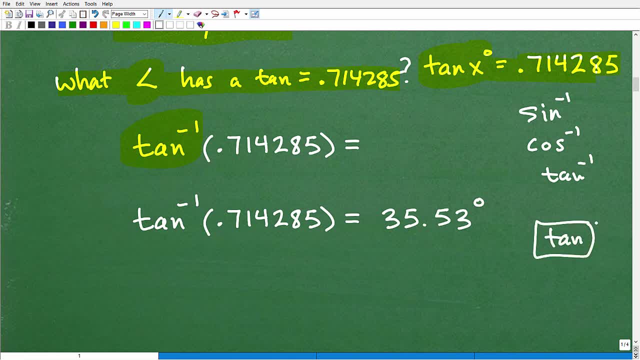 is on your calculator, you're going to have a tangent and then you're going to have a tangent, you'll have a tangent button. but you also have a second function on your calculator and if you look like here's your button, uh, on that, like the face of the calculator, you should, you should see. 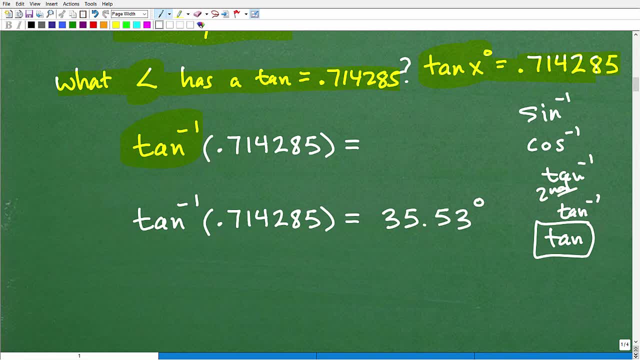 something like this. okay, so you'll have to kind of play with your calculator. you can use these. uh, use this here as an example to know how to use it. so if i plug in or if i hit the second function and i bring up arc tangent, this guy right here and i put in this decimal, okay, this is going to tell. 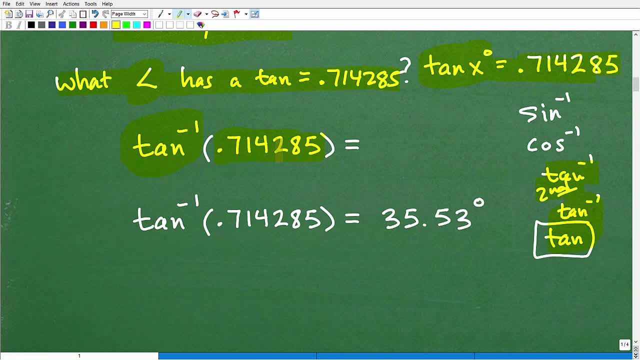 me that the angle has a tangent that's equal to 0.714285, so i plug this into my calculator. by the way, it's very important that your calculator is in degree modes. we want our answer in degrees because you can have your calculator in radian modes, which will give you a different answer. 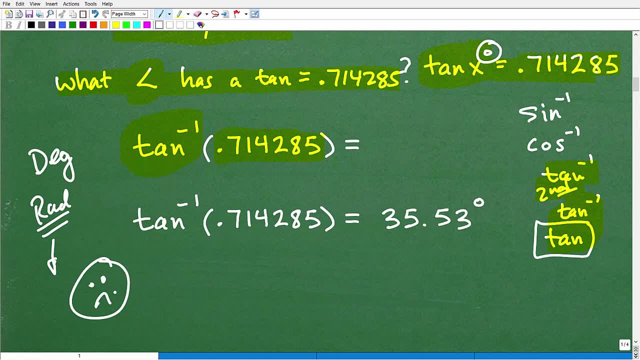 and then you'll end up with one of these, these little sad faces, and that's not good, okay. so when you're working in degrees, you'll have to put your calculator make sure it's in degree mode. it should be in degree mode by default, okay, if it's in radians, that means 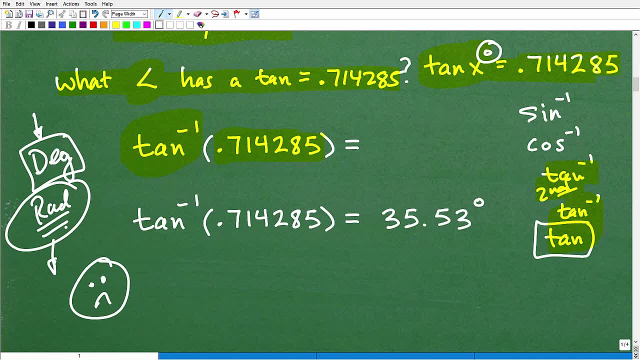 you're kind of messing around now. you'll also need to know how to work with radians, but that's for different topics. so just make sure your calculator is in degree modes, because our answer is going to be in degrees. okay, so we're going to plug this into our calculator. it's not the tangent. 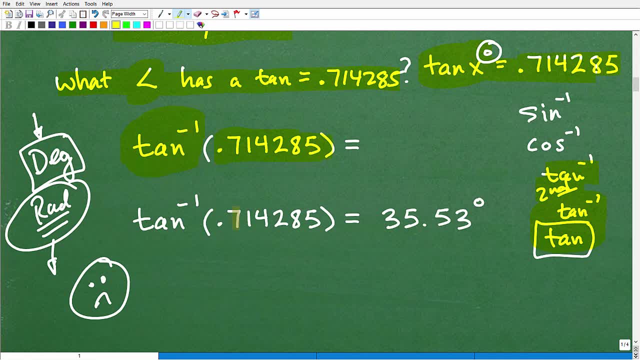 it's going to be the arc tangent, this tan negative one. you plug in your decimal, just like this, and you hit enter and this pops out again: I'm rounding, but you're going to get 35, 0.53 degrees. okay, that's a little degree sign right there and that is the answer. okay, 35.53. 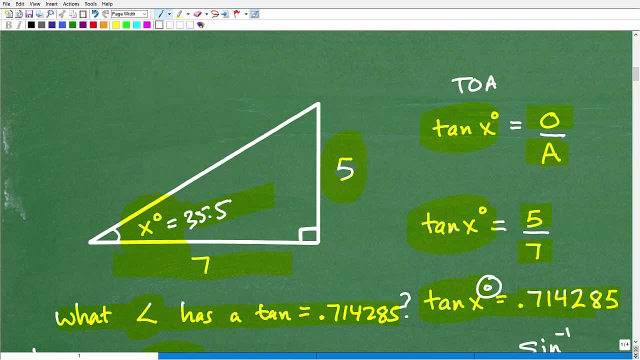 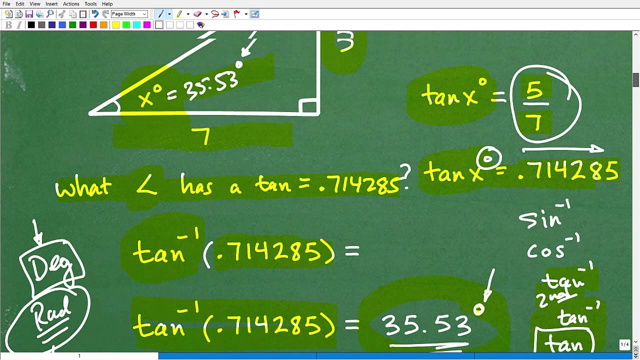 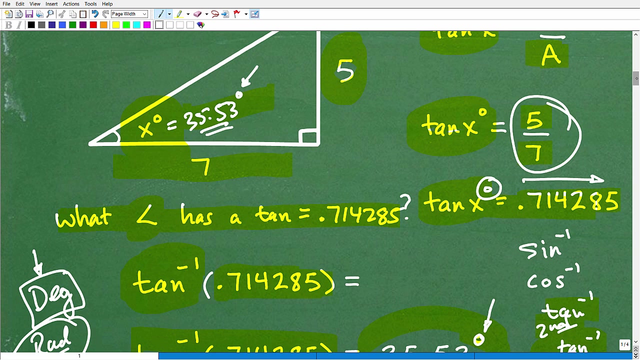 right here: 35.53 degrees. okay. now, the more digits I use in terms of of calculating 5 over 7, the more accurate this becomes okay. so you just need to know that as well. so you don't want to round off, the answer won't be as accurate. but this process here, this is how you find angles of right triangles. 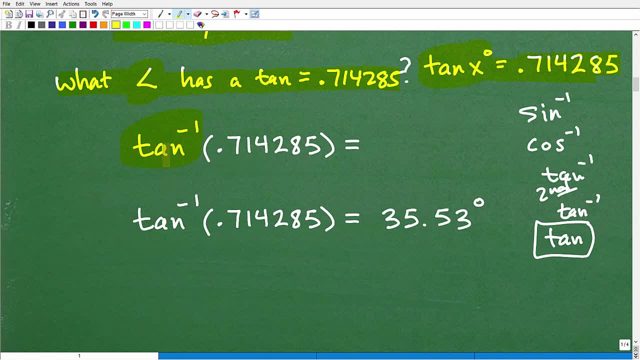 use this here as an example to know how to use it. So if I plug in or if I hit the second function and I bring up our tangent, this guy right here and I, uh, put in this decimal. okay, this is. 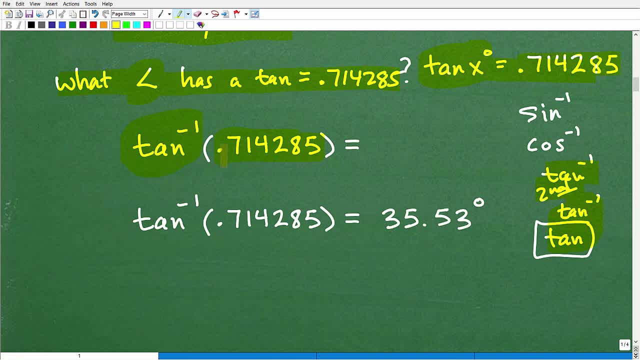 going to tell me what angle has a tangent that's equal to 0.714285.. So I plug this into my calculator. by the way, it's very important, uh, that your calculator is in degree modes. We want our answer in degrees because you can have your calculator in radian modes, which 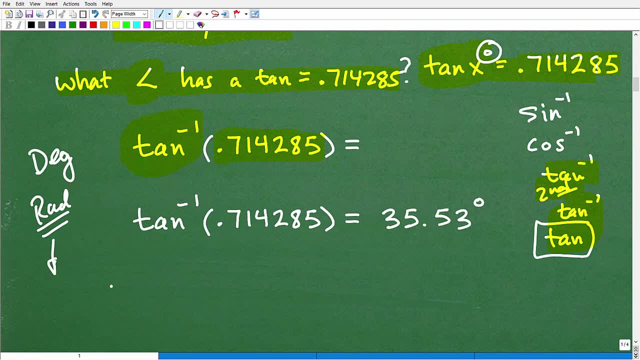 uh will give you a different answer, And then you'll end up with one of these, these little sad faces, and that's not good, Okay. So when you're working in degrees, you'll have to uh, put your calculator make sure it's in degree mode. It should be in degree. 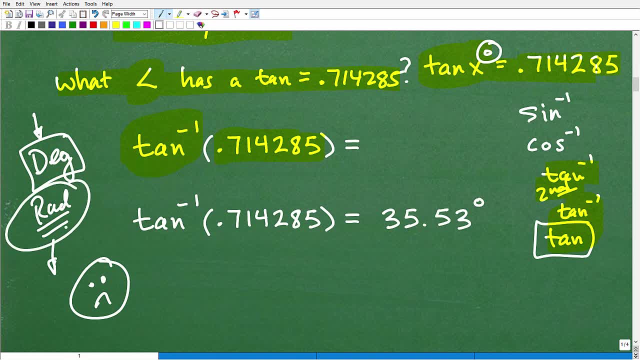 mode by default, Okay, Um, if it's in radians, that means you're kind of messing around. Now you'll also need to know how to work with radians, but that's for a different uh topic. So just make sure your calculator is in degree modes, because our answer is going to be: 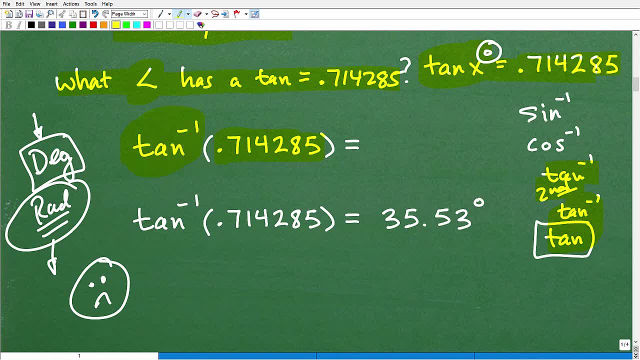 in degrees. Okay, So we're going to plug this into our calculator. It's not the tangent, It's going to be the arc tangent, this tan negative one. You plug in your decimal, just like this, and you hit enter And this pops out again: I'm rounding, but you're going to get 35.53. 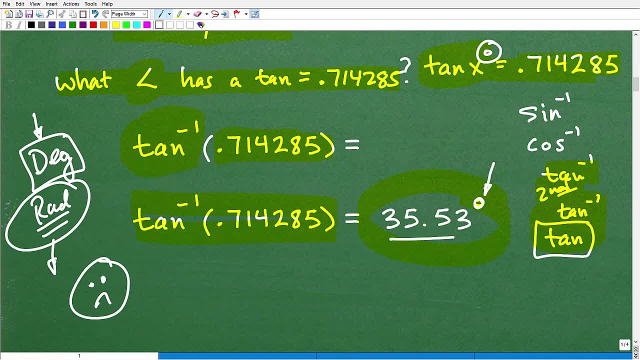 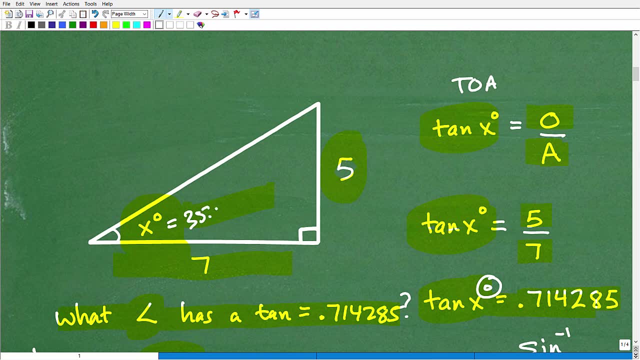 degrees. Okay, That's a little degree. uh, sign right there And that is the answer. Okay, It's 35.53, right here, 35.53 degrees. Okay, Now the uh more digits I use in terms of of calculating five over seven. 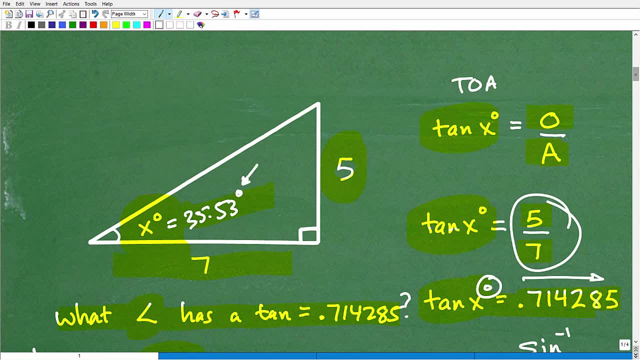 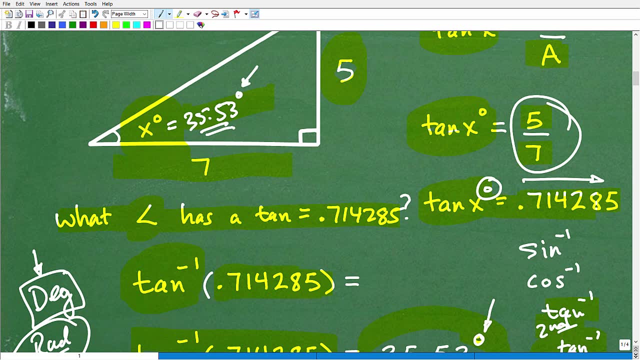 the more accurate. uh, this becomes Okay. So you just need to know that as well. So you don't want to round off too much. You don't want to use 0.7, because this answer won't be as accurate. 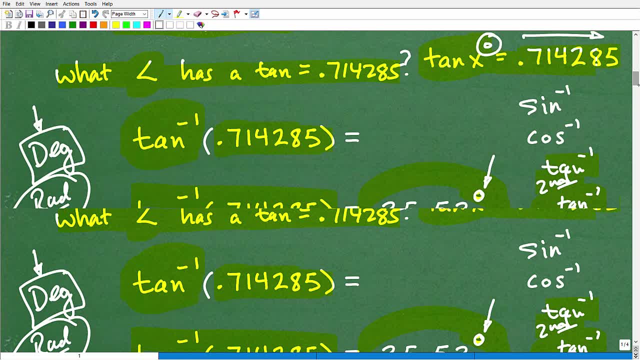 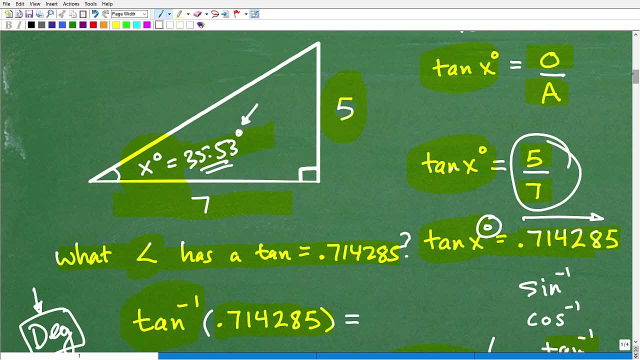 but this process here um, this is how you find um angles of right triangles. There's some, there's some kind of special case Techniques, but this is basic trigonometry. Okay, Using a basic trigonometric ratios that 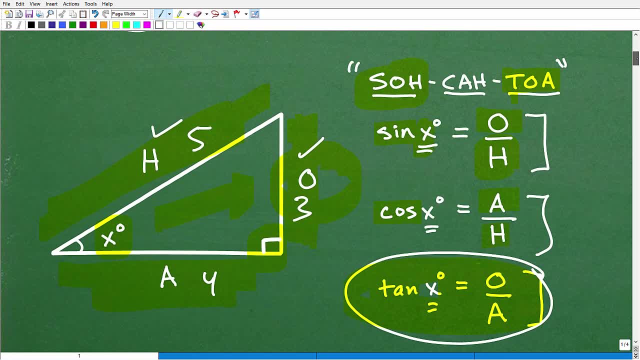 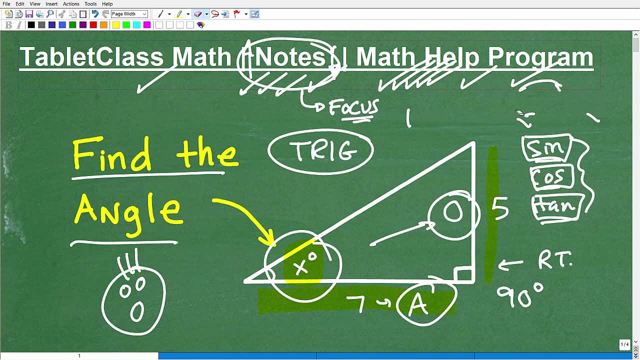 we just kind of covered. So if you've never taken trigonometry or you didn't know anything about it, well, this is a good little introduction to you. And uh boy, look what a mess I made over here, Let's go and erase this here. So we kind of uh think, now what do you study? 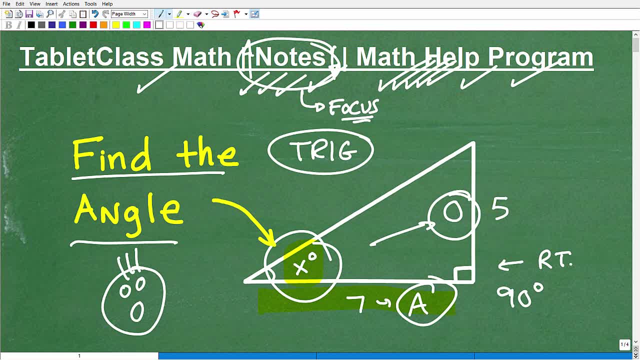 trigonometry, All right. Uh, if some of you are out there like: well, when, when am I going to see this? Well, typically you'll start studying basic trigonometry and geometry. Okay, That's pretty common. But then when you move on to uh courses- like there's some courses- 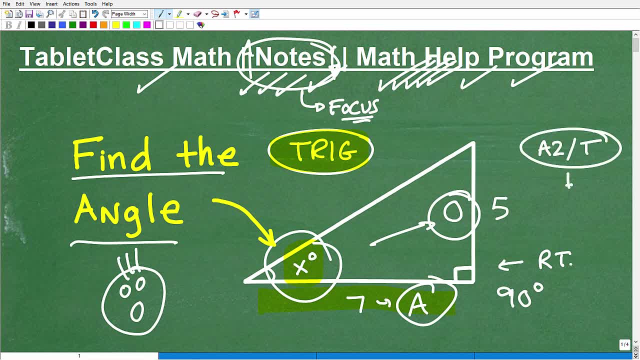 called algebra two trigonometry, but typically this is uh more or less uh covered in like a pre-calculus course. Okay, That's uh really when you're going to uh get into it, but this: 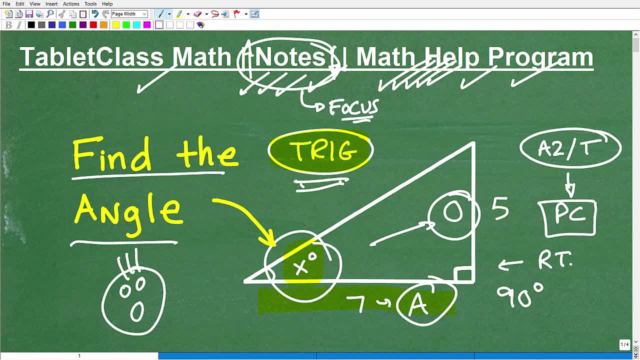 basic trigonometry stuff you will see in geometry, at least most high school level uh geometry courses, Okay. So if this video was interesting and now we know, hopefully we're not scared of this anymore. We have a happy face, If you like this. 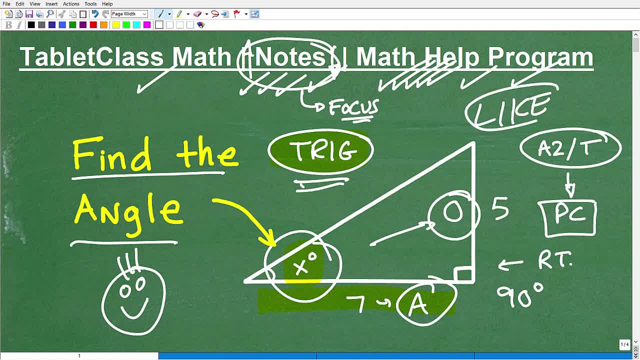 video, uh, and you're like, oh yeah, this was useful. Well then, please consider smashing that like button And if you're new to my YouTube channel, please consider subscribing. Been on YouTube for a long time, Um 10 plus years. I know I have over a thousand videos. I stopped counting. 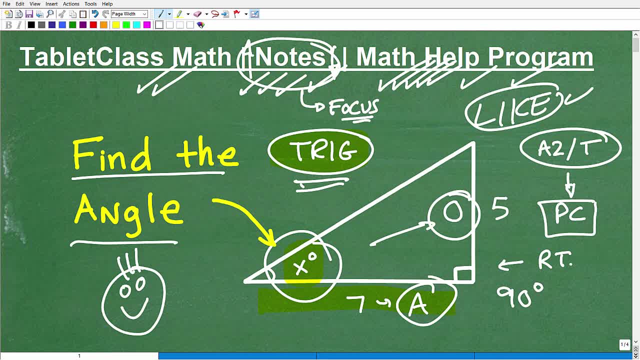 my job. What I'm focused on is trying to teach math in a clear and understandable way. That's my mission, And nobody should be failing math. Okay, Uh, you know, if you're failing, if you're struggling, you're going to fail. So if you're failing, you're going to fail. So if you're. 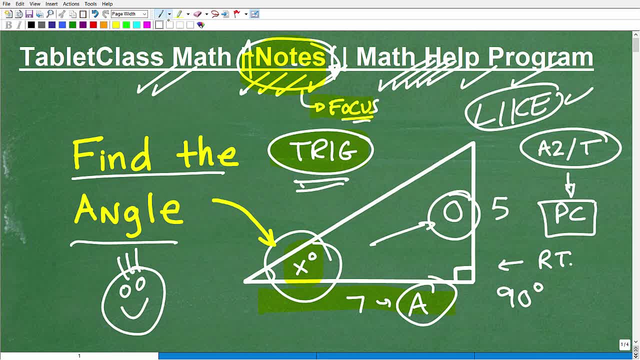 failing, you're going to fail. So if you're failing, you're going to fail. Take a look at your notes. improve, uh, your note taking and then talk to your teacher. get more help, but you're going to. 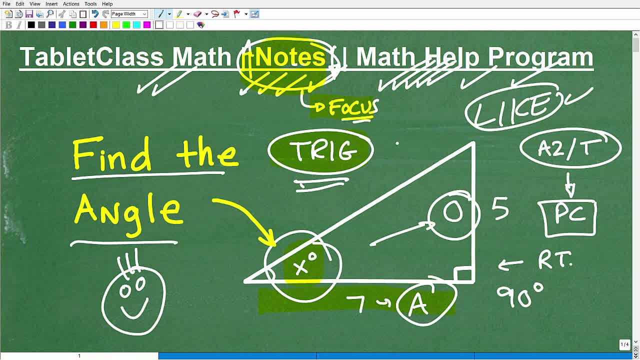 have to take the initiative right. Go out and find instruction that you like. If you like my teaching style, then I have tons of videos organized on my playlist there. You can just, you know, learn about a lot of different topics, but my best math help will always be in my math. 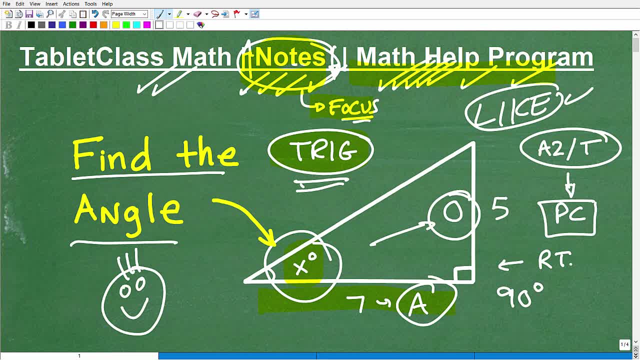 help program. Okay, So with that being said, I definitely wish you all the best in your mathematics adventures. Thank you for your time and have a great day.